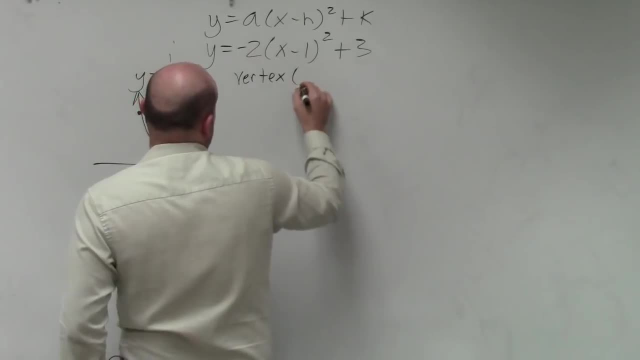 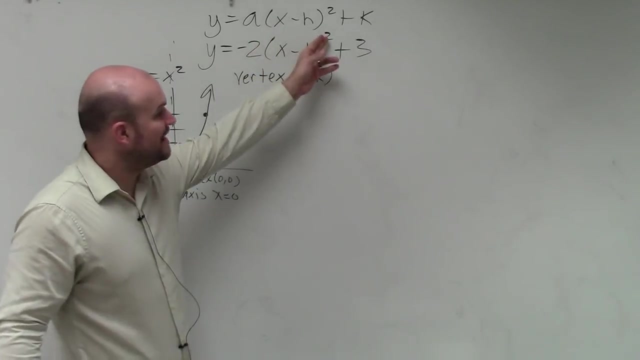 quickly identify the vertex. The vertex in this case is going to be h comma k. So remember it's x, x opposite of h. So in this case it's x opposite of 1.. So you can say that h is equal to. 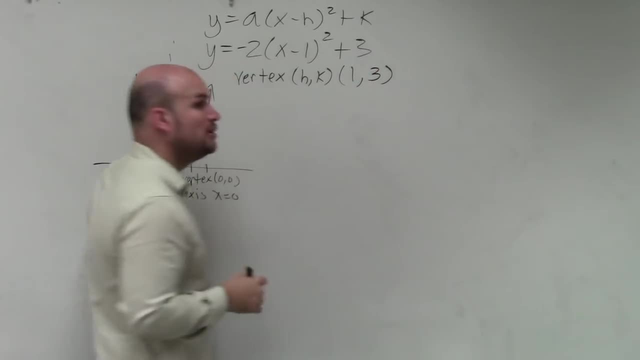 1, and your k is equal to 3.. So my new vertex, instead of being at 0, 0, is now at 1, comma 3.. So I'm going to basically take my vertex, which is here, and go over 1, and then up 3. 1,. 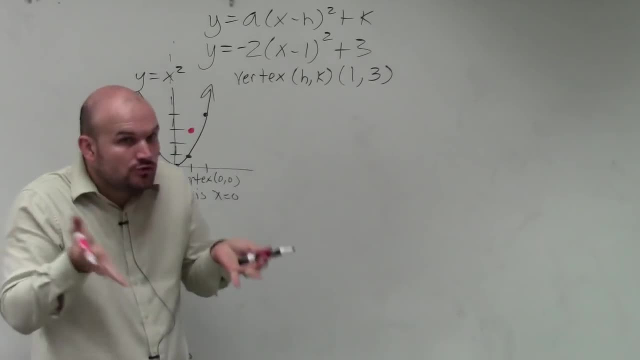 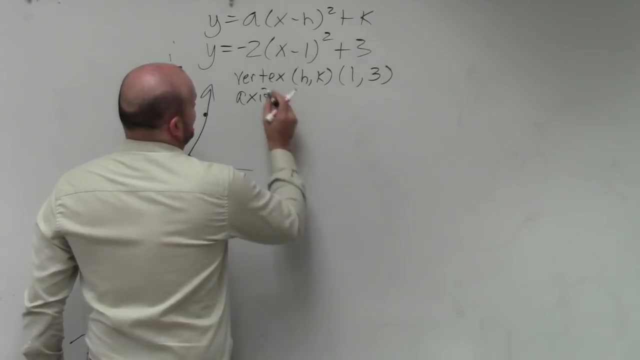 2,, 3. And make a nice big dot. That is my new vertex. Does everybody follow me with that? The axis of symmetry, when in vertex form is x equals h. So since we know that my h is 1,, 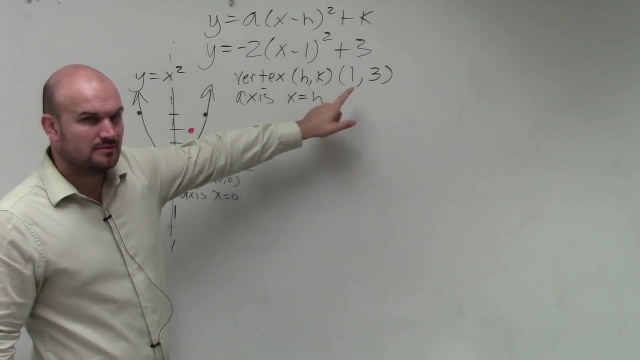 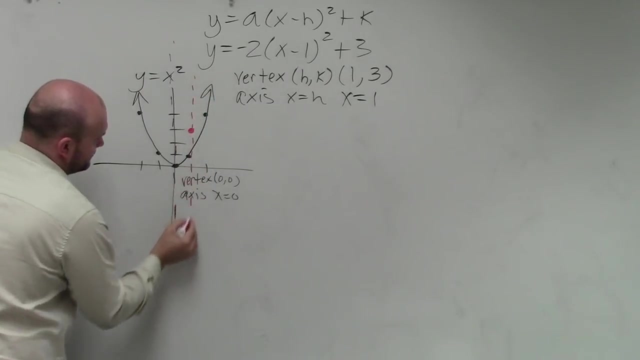 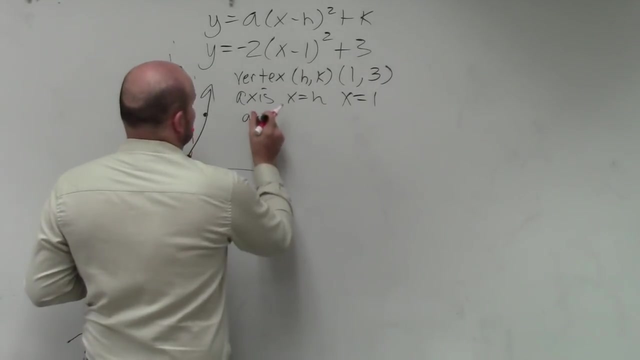 does anybody have any questions why it's 1 and not negative 1? No, OK, So I'm going to take my vertex and I'm going to say h equals 1.. So then I go over to 1, and draw a nice little dotted line. OK, Also, in your notes we talked about a When a is less. 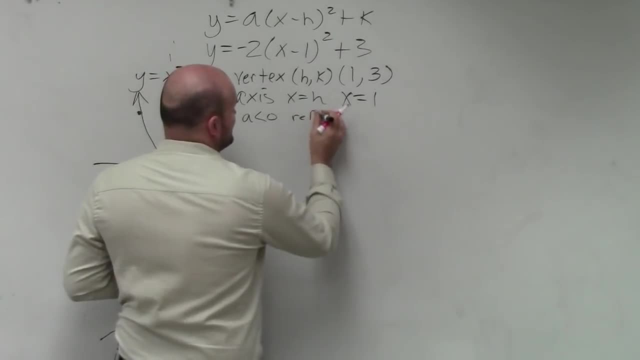 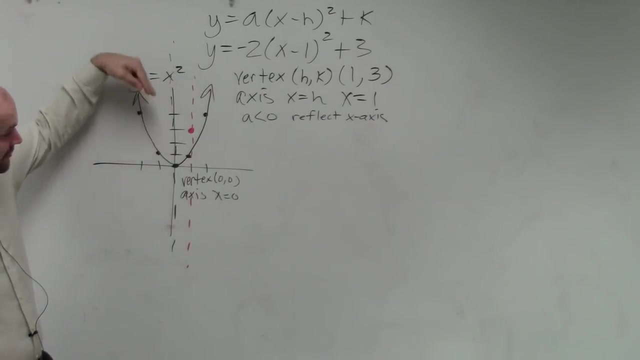 than 0,. this is just replaying your notes. you reflect the x-axis, So, rather than the graph going up, now the graph is going to face down. So I'm just going to draw two little arrows just to remind myself that the graph is now going to be facing down. 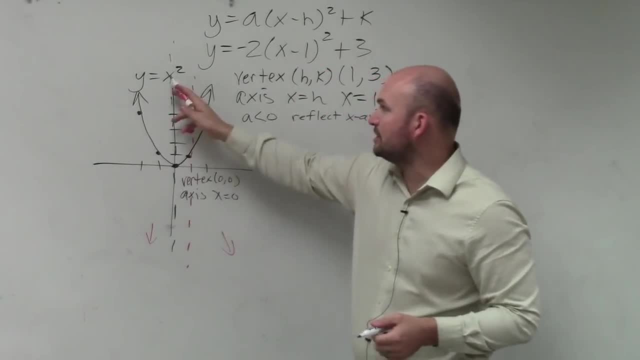 If you look at the paragraph, remember, this graph comes in If I plug in 1 here, 1 squared is 1.. 2, 2 squared is when you plug in 2, so you plug in 2 for x, 2 squared though. 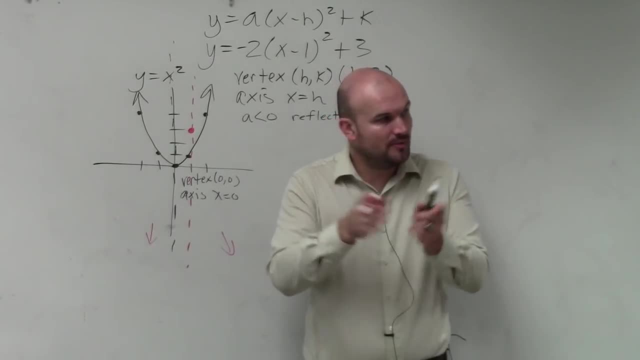 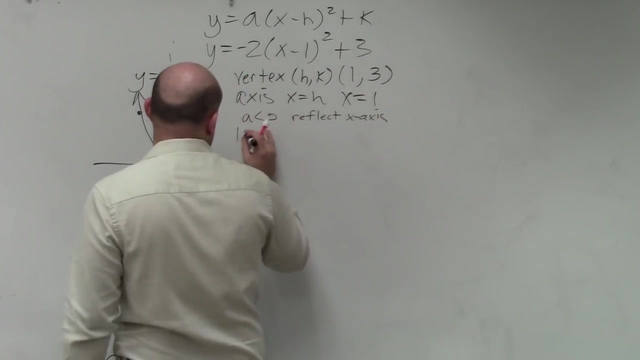 gives you 4.. So, instead of going, you're basically going over 1, up 1, over 2, up 4.. However, now I'm multiplying it by, I have a compression And, if you guys remember, when the absolute value of a is greater than 1, you have a. 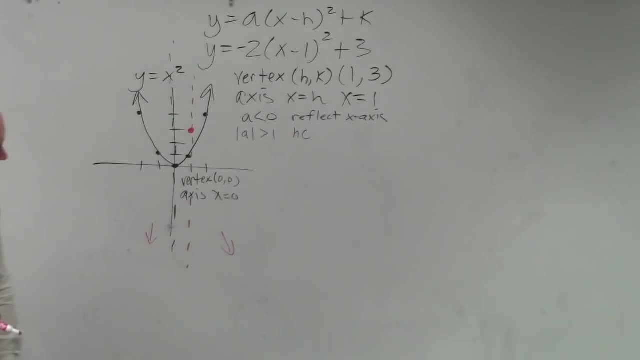 horizontal compression. I'll just write it as h2 to save some time. So basically, what that's doing is all that number 2 is doing is when you go over 1, when you plug in your x, then you have. 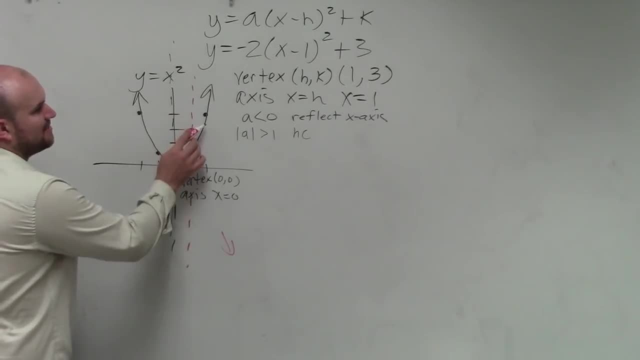 to multiply that by 2.. So let's see what happens. Let's see what happens with this. When I go ahead and go over 1,, typically if there was a was 1, I'd go over 1,, down 1.. Over 1,, down 1. I'd follow. 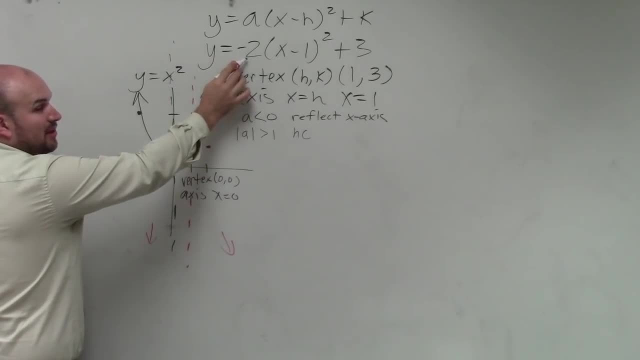 this real force, but I'm going down instead of going up. But now I'm multiplying it by 2.. So I'm going. once I square that, I'm going to go down 2.. Left 1, down 2.. And you can always. 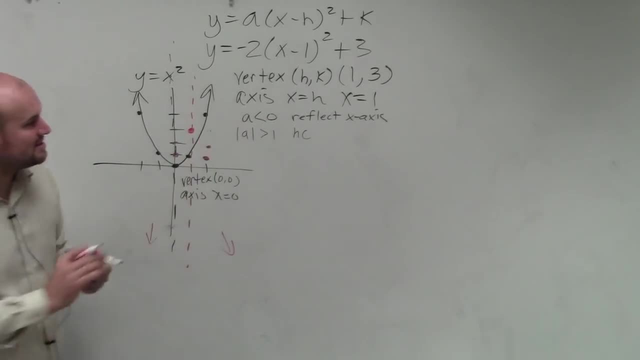 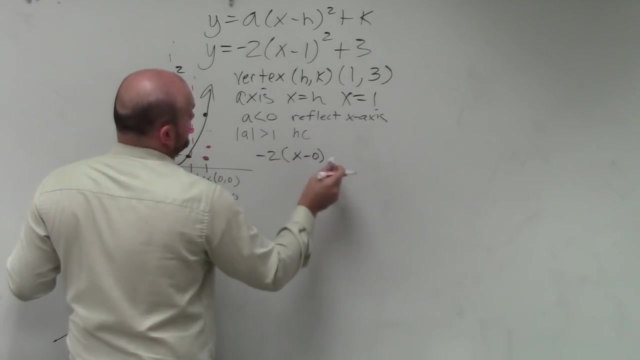 check your answers, ladies and gentlemen, by just plugging in points. If you know here is your value, let's figure out what 0 would be So negative 2 times x minus 0.. Oops, I'm sorry, Yep, no, 0 minus 1 squared plus 3.. So if you plug this in, you get 0 minus 1. 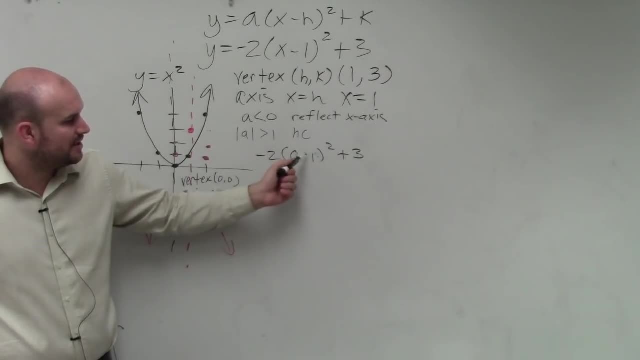 is negative: 1. Negative 1 squared is Negative. 1 squared is 1.. 1 times negative 2 is negative 2. Plus 3 is actually negative 1.. So actually, I'm sorry, I didn't follow my rules. If you plug that in your point actually now becomes. 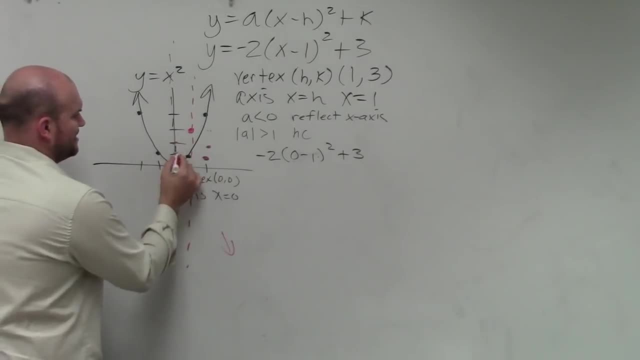 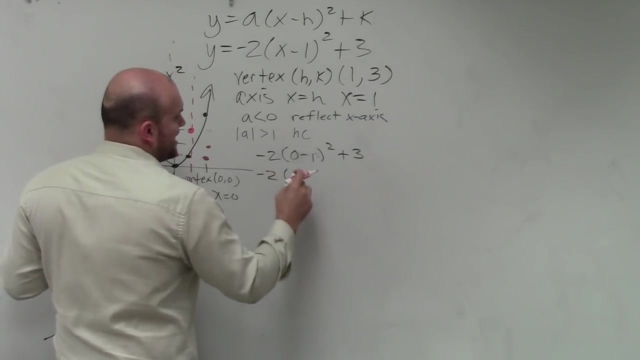 0, 3.. Oh yeah, it is 1.. I was right, I did, It is positive 1.. So now let's pick another point. Let's pick negative 1. Negative 2 times negative: 1 minus 1 squared plus 3.. Negative 1 minus 1 is: 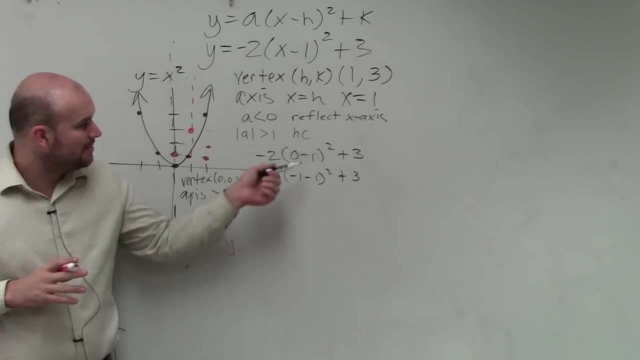 negative: 2. Negative 2 squared is going to be negative: 1 minus 1 squared plus 3. Negative 1 squared is going to be positive. 4. Positive 4 times negative: 2 is negative. 8. Negative 8 plus 3 is negative, 5. So 1, 2,, 3, 4, 5. So at negative 1, I'm going down to negative. 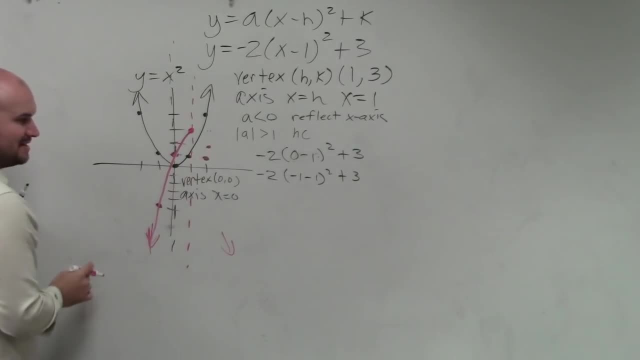 5. Basically, you guys can see that this graph goes like this, And then all you simply need to do is with the axis of symmetry. you just reflect the points across the axis of symmetry. I don't know why my graph looks off. in that case. The point should be over. Oh, that's a little bit.